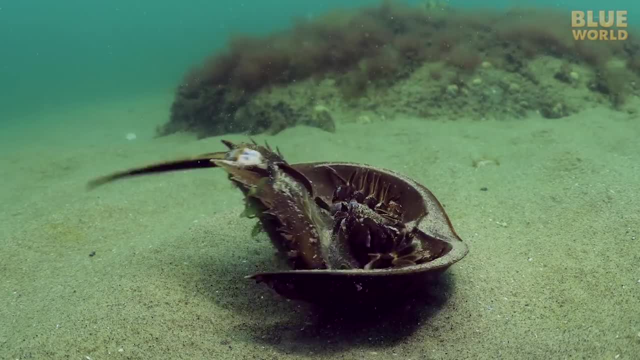 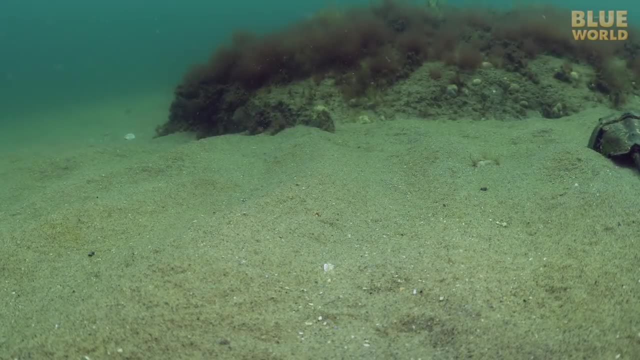 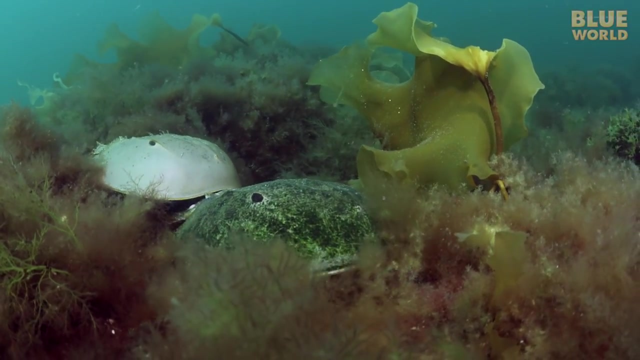 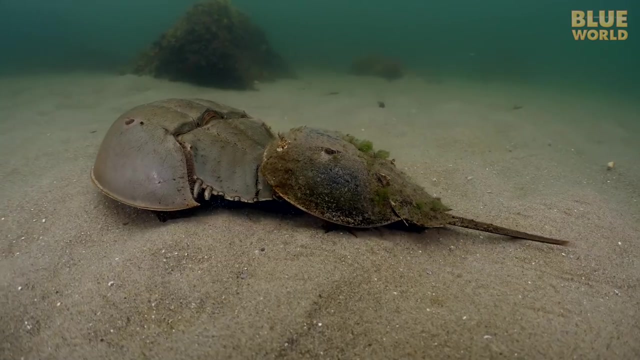 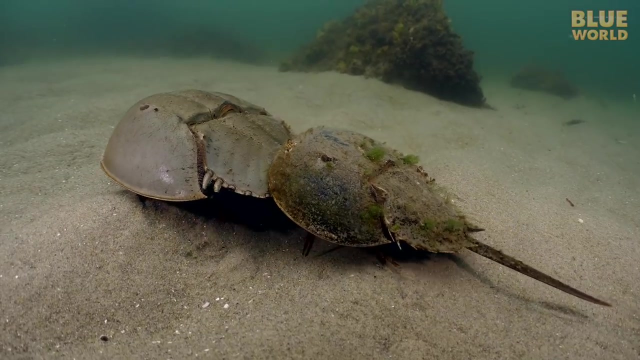 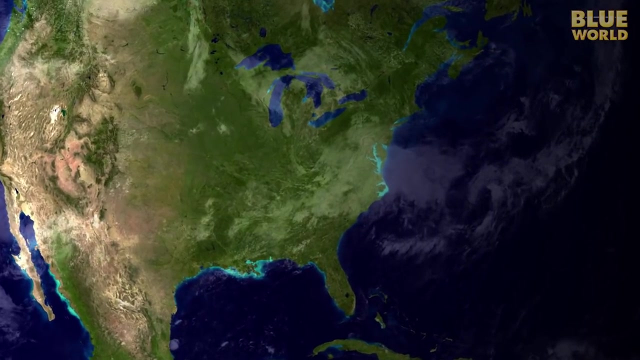 But actually it has a much more more practical use. During the summer, when the water warms up, the mating season begins. Males hang on to the females and follow them everywhere until they're ready to mate. One of the biggest spawning aggregations of horseshoe crabs in the world takes place in the waters around Cape Cod. 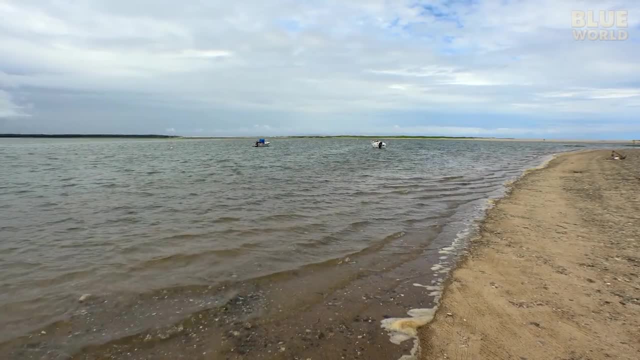 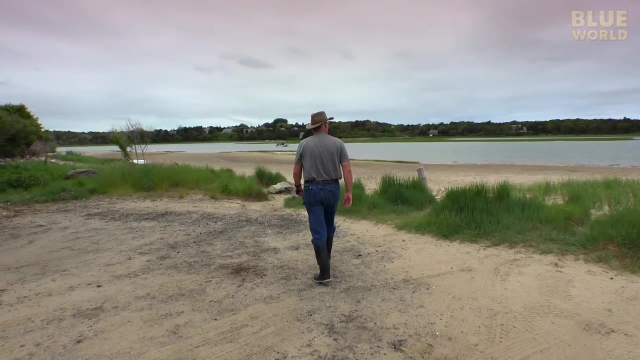 Because Cape Cod is basically a huge sandbar. it's shallow and sandy, perfect habitat for horseshoe crabs. I'm sending cameraman Tim on his first assignment as Blue World. I'm sending cameraman Tim on his first assignment as Blue World. 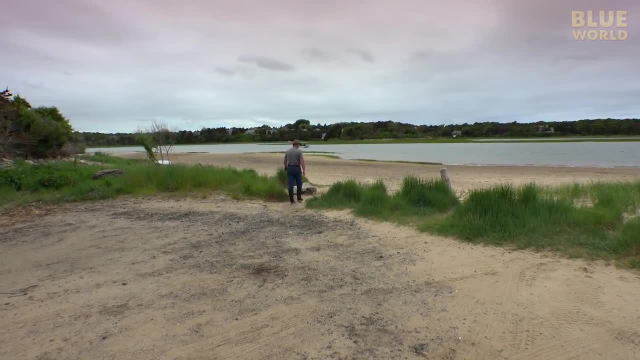 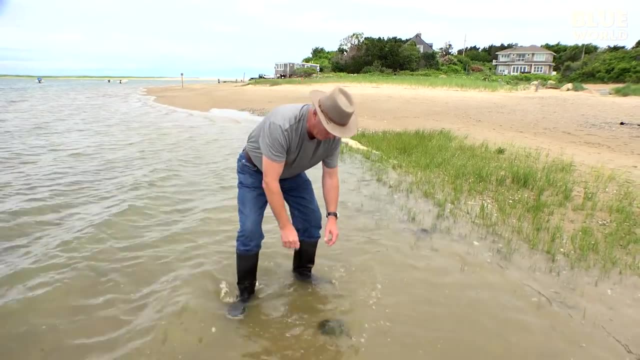 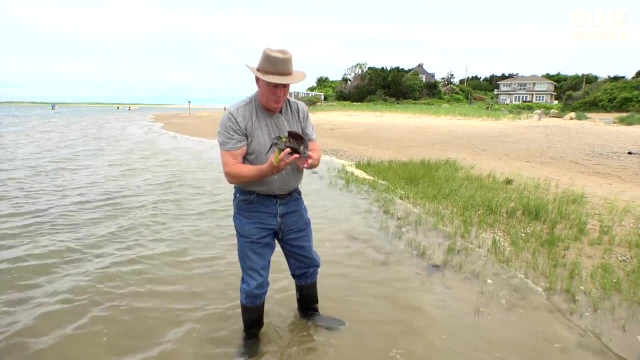 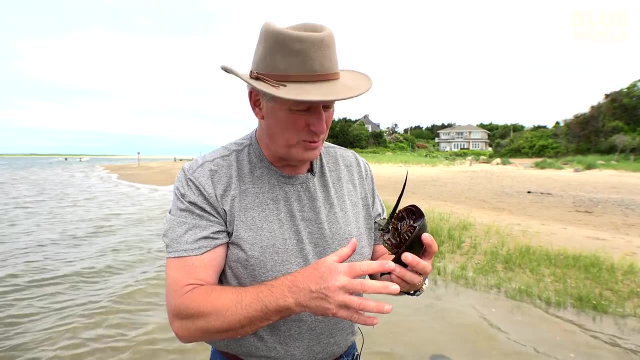 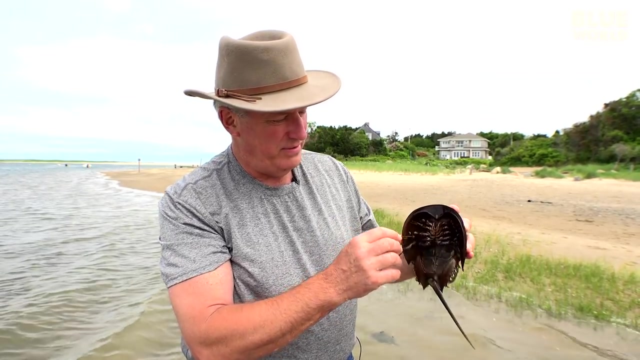 Tell me, if you can, What this? If you could tell me what this reminds you of This horseshoe crab. its ancestors go back almost 450 million years. What a fascinating little animal. If you look underneath, he's got all of his. 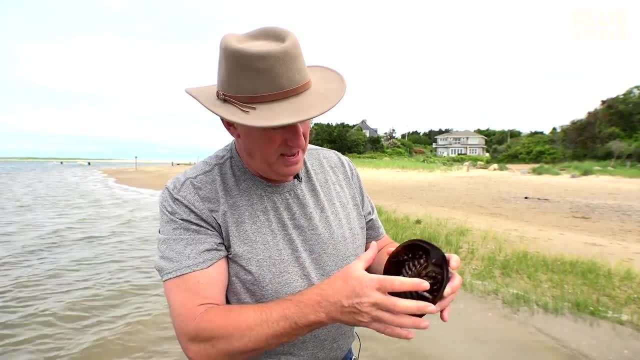 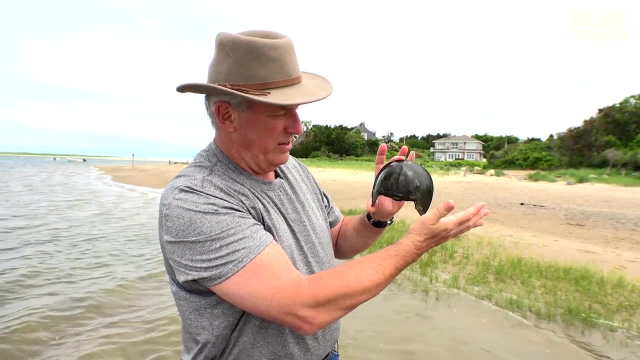 He's got 10 legs, his mouth- and this is the reason he's called a horseshoe crab- is because his shell, the head shell, looks like a horseshoe. He's got two eyes, two compound eyes on the front. He is not happy that I'm holding him. 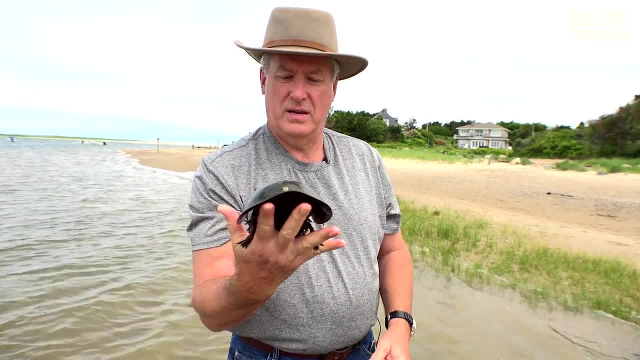 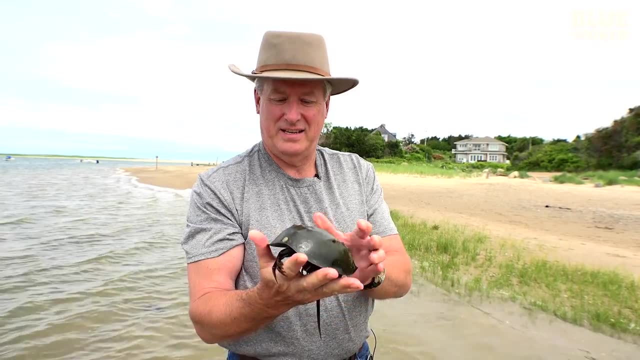 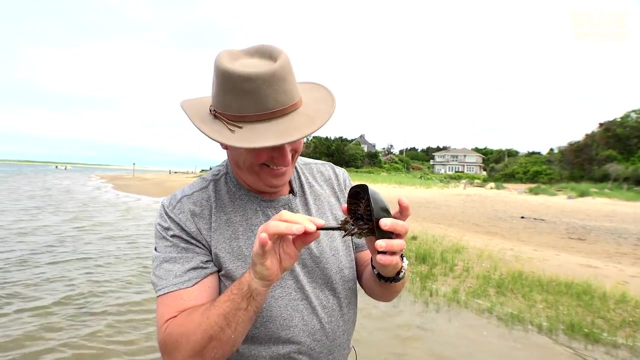 He's come up onto the beach because all the horseshoe crabs, they're all starting to breed and mate on the beach and lay eggs. Look at him. What does he remind you of? What movie Fascinating. I'm going to let him go. 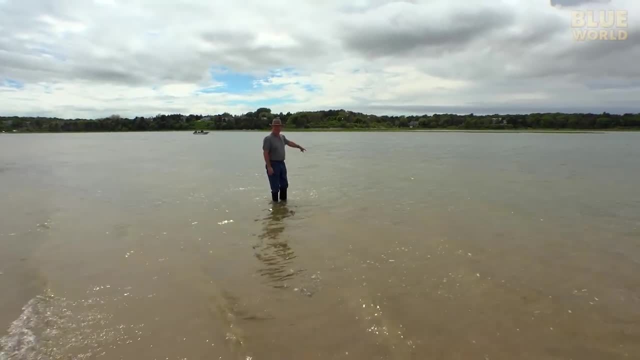 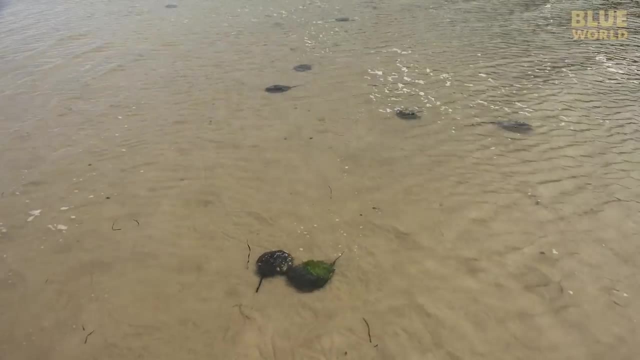 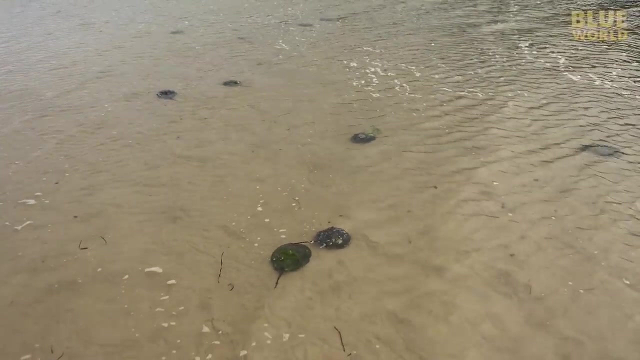 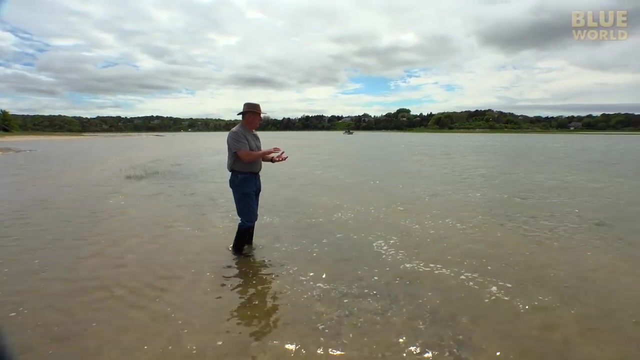 Yeah, there's a pair. There's a pair coming in right now. You can see them. You can see them everywhere, Those little black shadows all in the shallow water here right now And they're all coming in. They have one male on the back of a female and they're all headed into the shallow water. 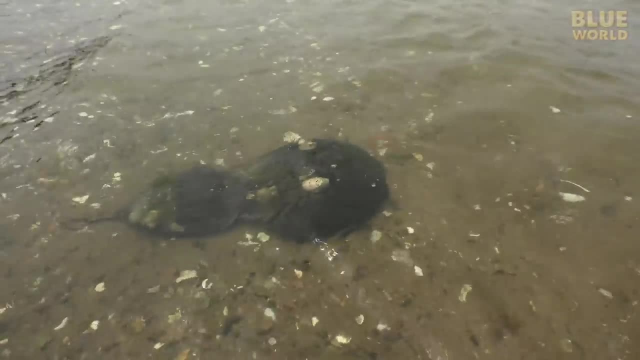 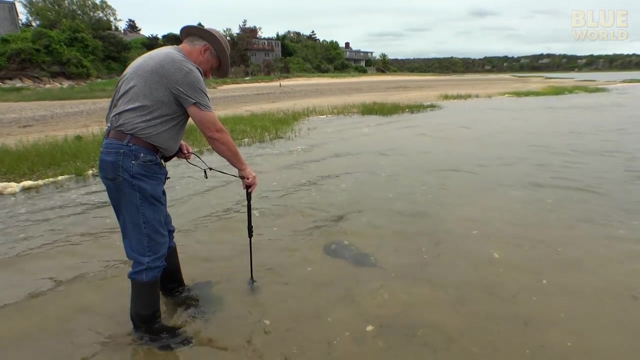 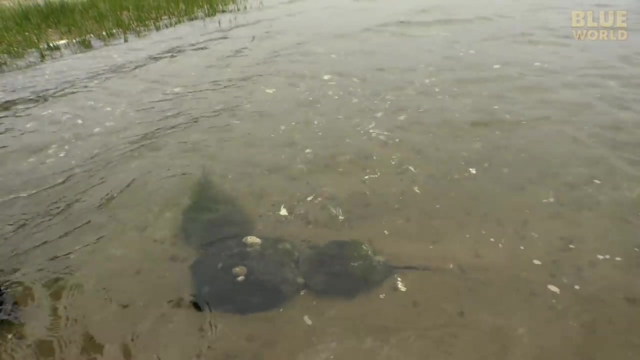 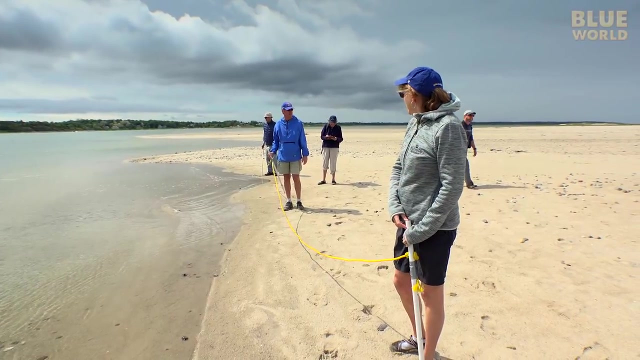 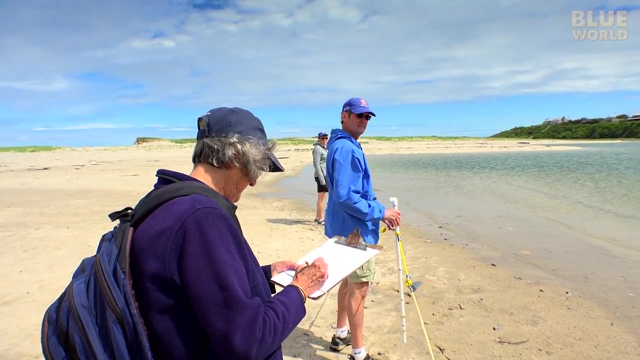 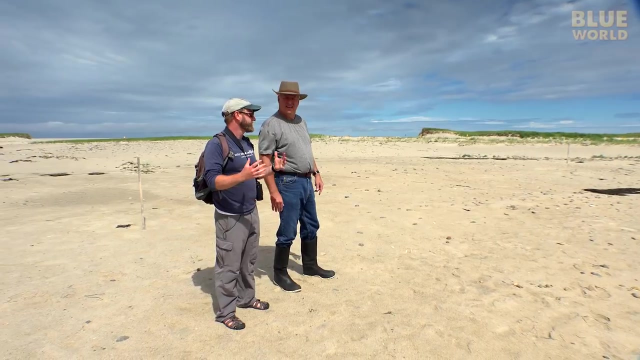 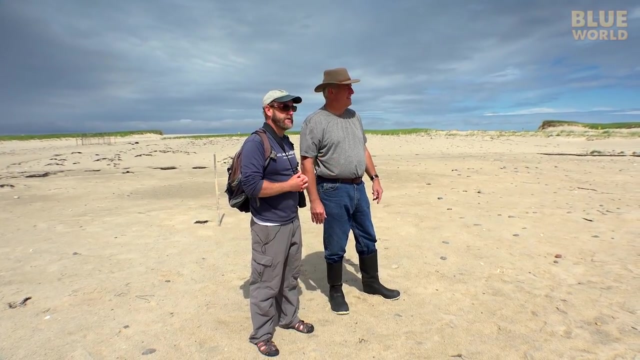 To learn more about the horseshoe crabs. Tim is meeting up with volunteers from Mass Audubon's Wellfleet Bay Wildlife Sanctuary, along with science coordinator Mark Faherty, So these guys are doing horseshoe crab spawning surveys, And so this is a standardized method used by organizations, volunteers, state agencies, federal biologists all up and down the East Coast. 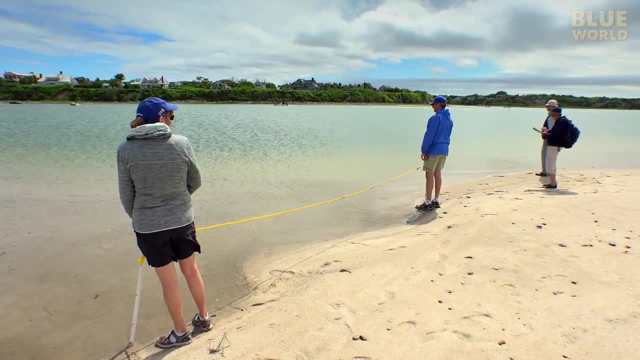 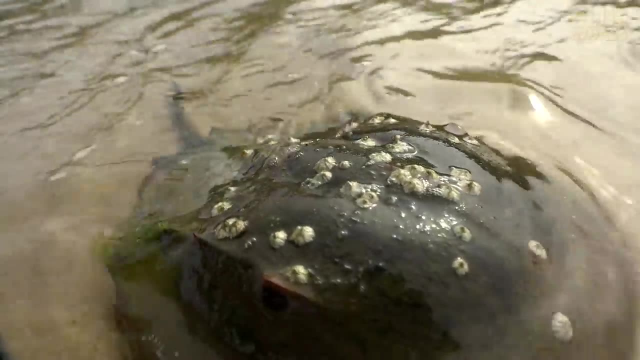 And the idea is these are five meter quadrats starting at the high tide line And it's just a standardized way to count spawning horseshoe crabs, Because horseshoe crabs come up to the to the water line on high tides to spawn. 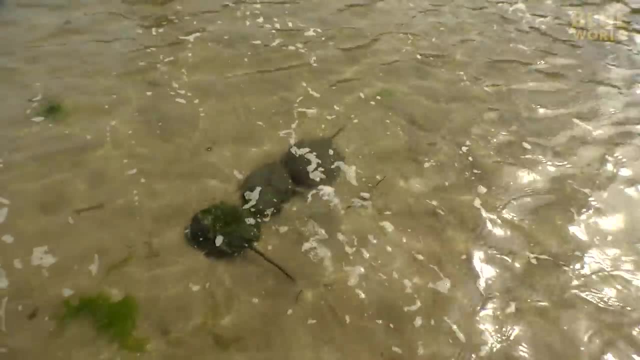 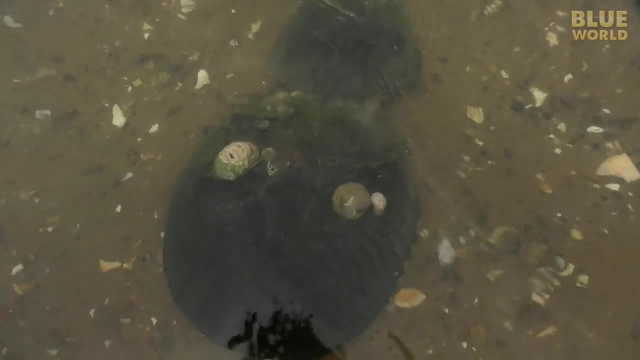 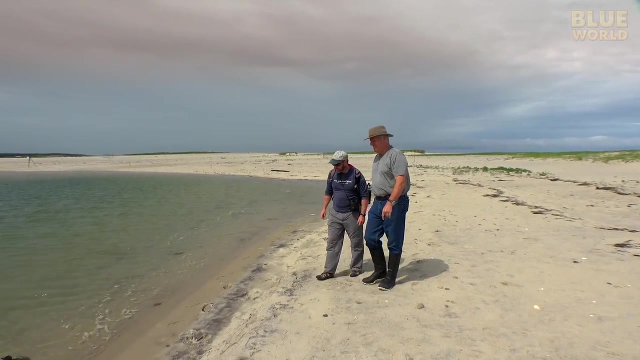 They spawn in the intertidal zone as well, quite a bit on Cape Cod. But this is the methodology that everybody uses, so the data is comparable across sites and across years. And yeah, here's some action right in front of us here. Look at that one. That one has like a muscle farm growing on her back. 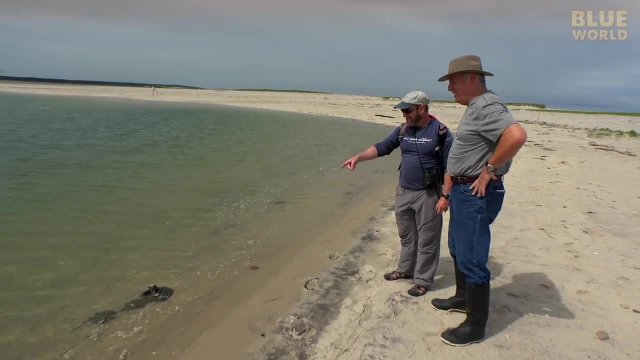 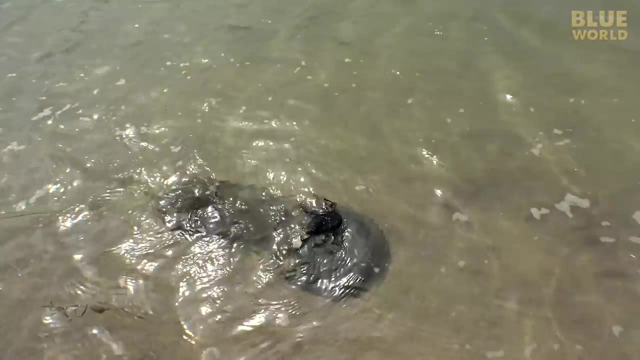 She's obviously hasn't been moving quick enough. The other They're holding on for dear life. Look at, one's got the tail. This is the end of the spawning season. I don't think this is the A-team here. Oh, wait a minute, That one's tagged. 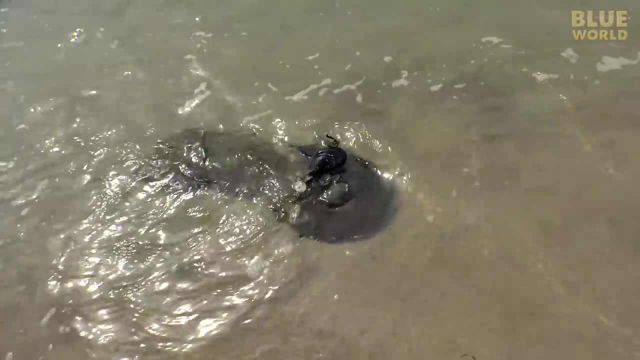 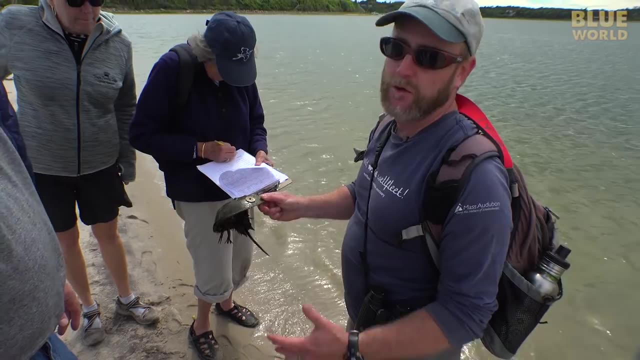 Did you guys read the tag off of this? Oh yeah, You got to check these guys for tags as you go. So this is a US Fish and Wildlife tag. We put it on, We do it. It's a great activity with school groups. 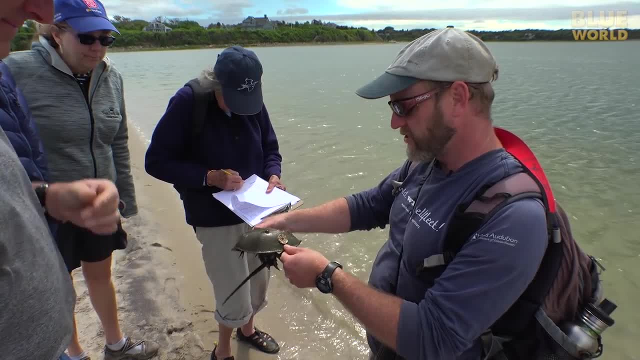 It's a great way to involve school groups in the research that we do. So this is a mark recapture project where you put a uniquely numbered tag on the crab. Yeah, So this is a mark recapture project where you put a uniquely numbered tag on the crab. 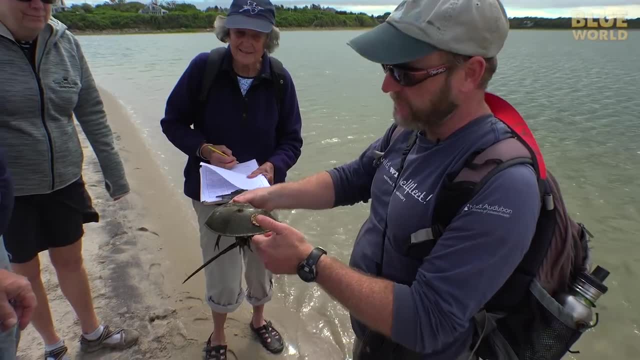 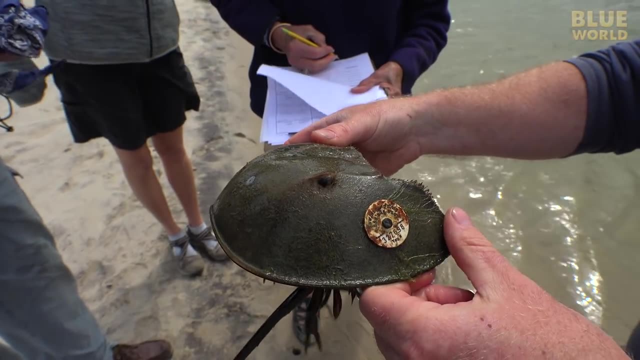 So this is a mark recapture project where you put a uniquely numbered tag on the crab and hope to find it again. So it gives you information on site fidelity. Do they come back to the same spawning site year after year? How much did they move around? 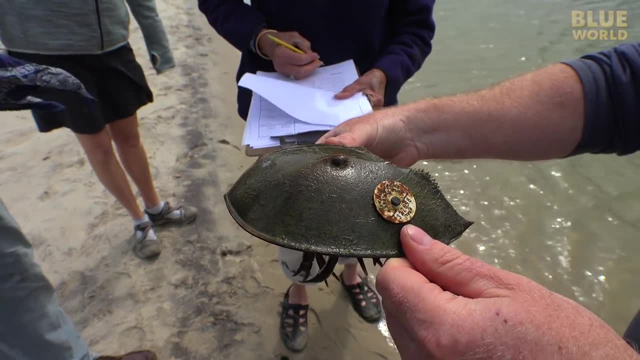 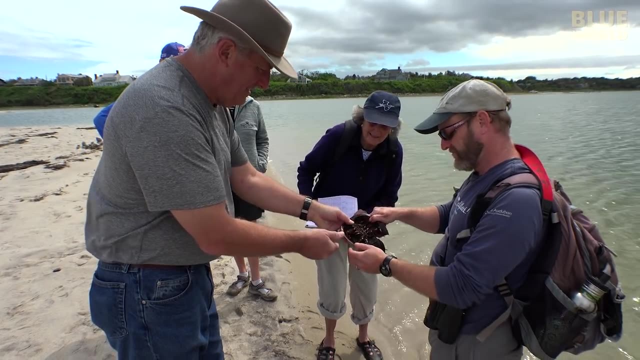 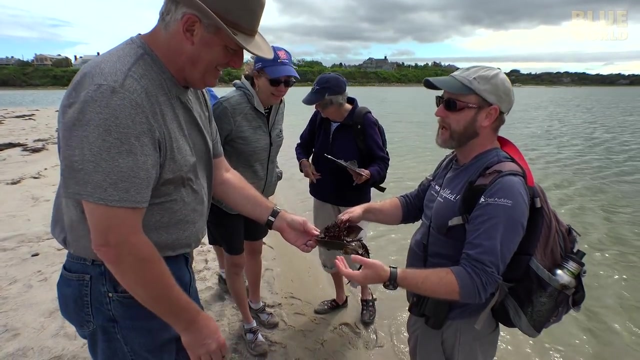 How long are they around, That, that kind of thing. And so this is a nice find, because we don't do a ton of tagging at this site. We do it sort of opportunistically. So this is a male, Yeah, And you can tell, because they have their front legs, have these boxing glove looking things called petty palps. 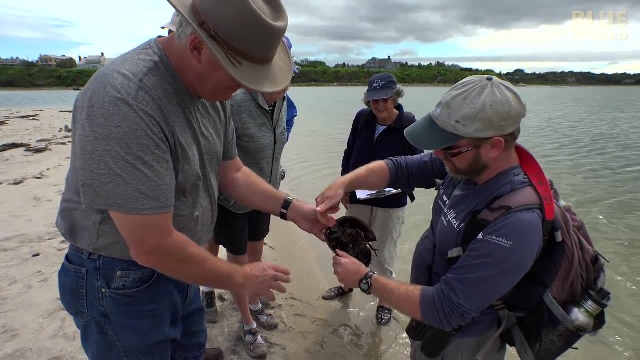 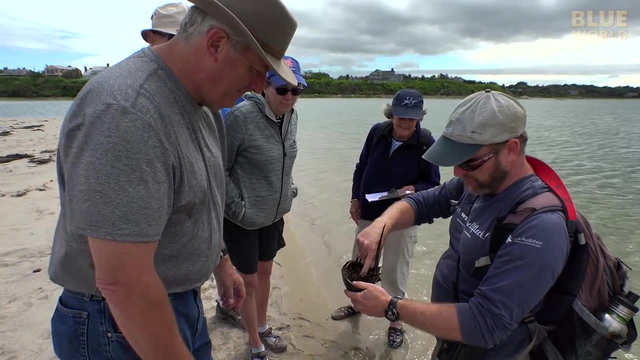 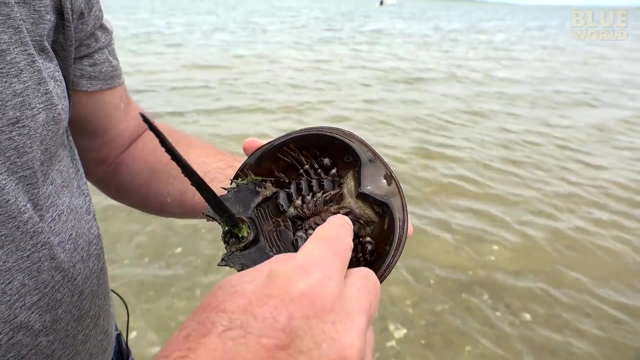 Yeah, And that's That's for holding on to the female. The males also have a really concave front of the shell for for kind of riding along the females back, and then their mouth is here at the base of the legs. They have these book gills, these flaps or their gills, and they haven't changed very much in four hundred and eighty million years. 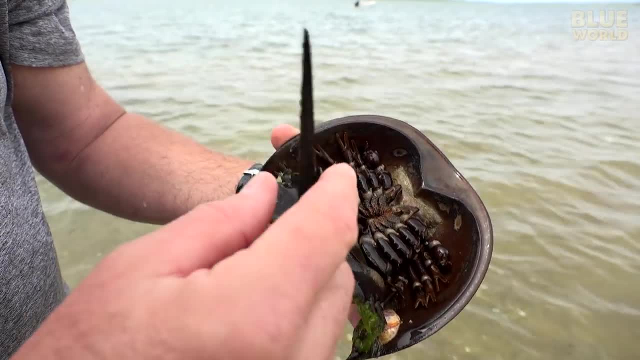 So I guess it works for them. We always tell people don't hold them by the Telson. Yeah, I'm sure there's kids out there like like me. when I was growing up at beaches in Plymouth thought it was a stinger, Yes, a stinger. 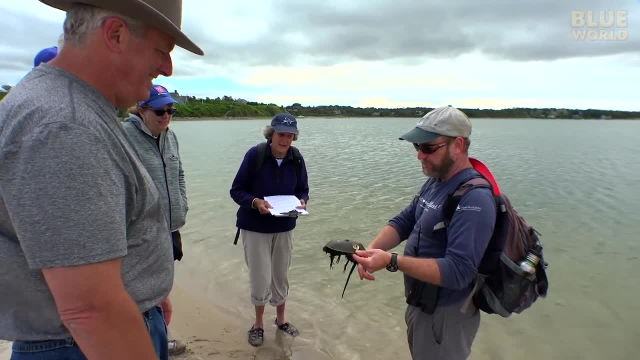 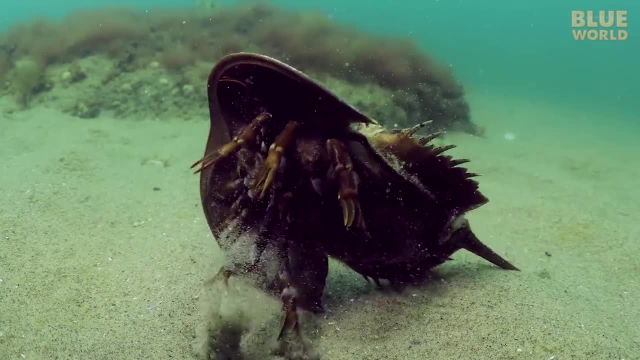 Watch out, But it's totally harmless by the tail. Yeah, Don't, don't pick them up by the tail. It's to help them because it can break off sometimes and it's critical for helping them flip themselves over if they end up on their back. 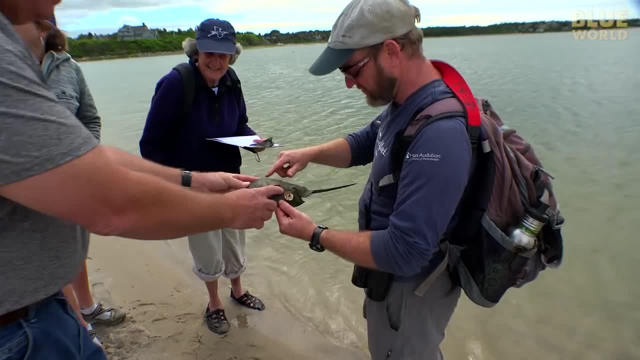 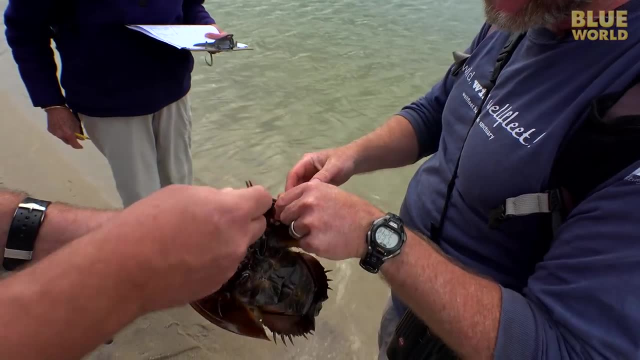 Yeah, And you know the eyes, Yeah, Yeah, Oh, they have all kinds of eyes. They have more than just these two. Yeah, I see them everywhere. They have light receptors, even on the Telson and underneath other places. There's one right there. 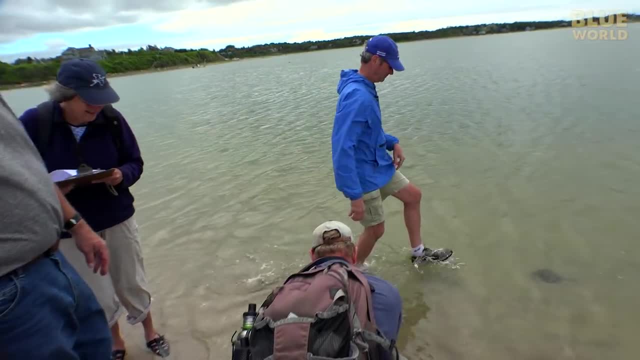 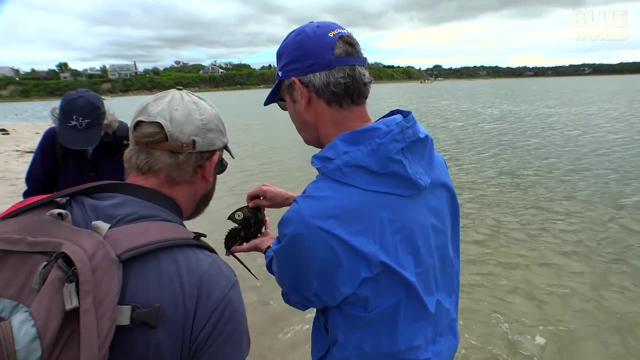 Look at this, Look at that. They're all got tags And I wonder I would. Oh my God, That's amazing. I should check to make sure they aren't the tags that we've had last time. All right, Let me know when you're ready. 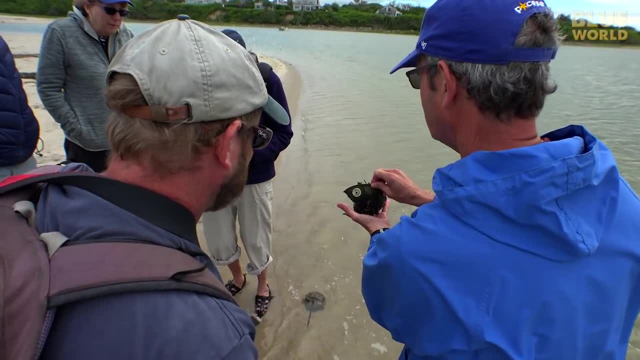 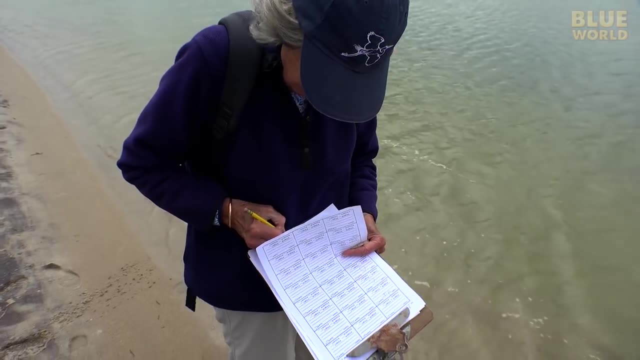 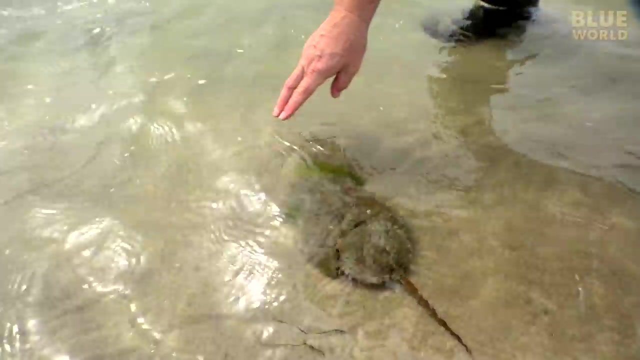 Almost a little cleaner. It does look newer. Okay, Three five, three. Three, five, three, Three, nine nine. This is what we came for right here. This is happening right now. Check it out. You can see this great big lump in the water. in the front is the female. 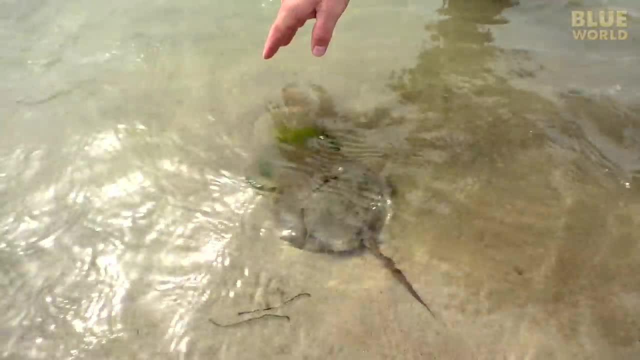 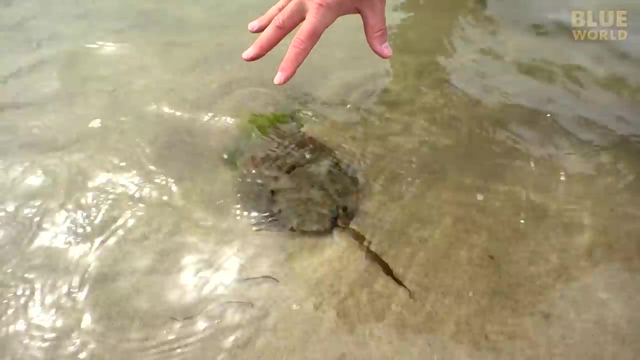 She's dug into the sand and she's laying the eggs right now. The male Who's Attached to her back, He is waiting for those eggs to go in the sand and he can fertilize them. She'll get up and she'll move along and she'll dig back down. 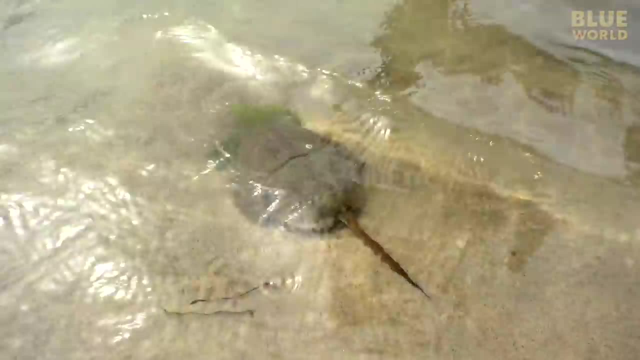 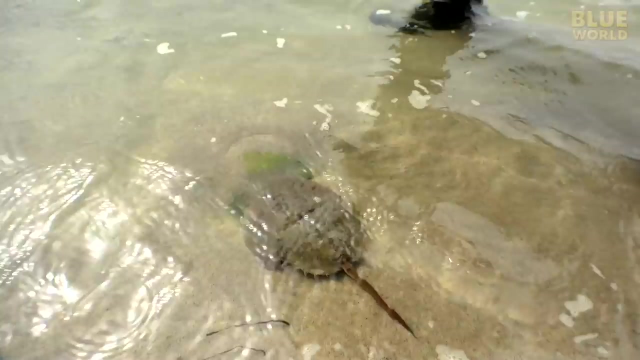 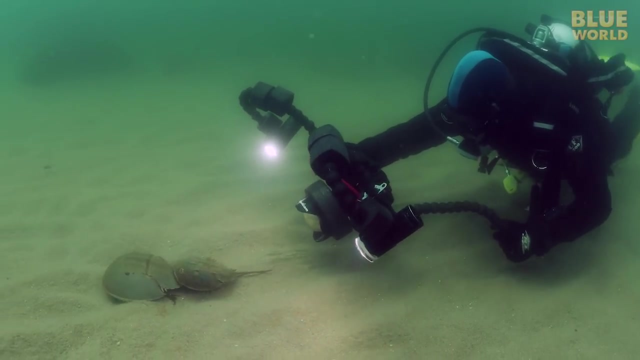 And I mean, this is what we came out here for- to see this And this is what the surveyors and Mass Audubon is looking for. is this little action right here? That's what it's all about. Horseshoe crabs are something I've seen on my dives here in New England ever since I first started diving.